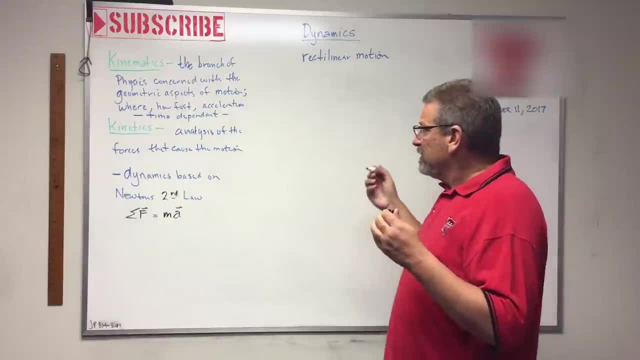 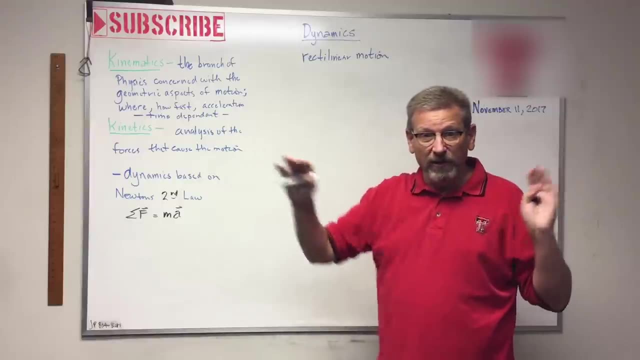 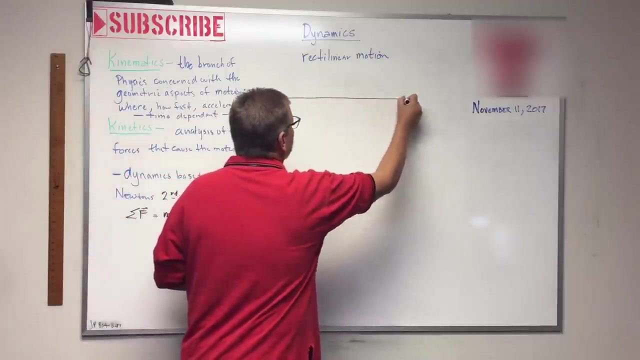 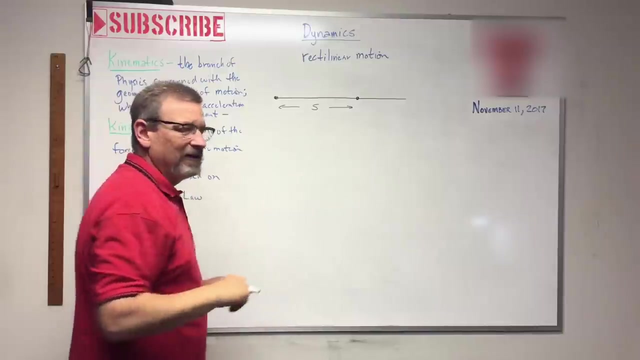 rectilinear motion. okay, so a particle is moving in rectilinear means, you know, just a XY direction, a linear direction. so let's just assume we have a particle, I don't know, that moves on a straight path, and there he is. okay, this is the distance, X, I mean, I asked rather- and S is just the location of that place in. 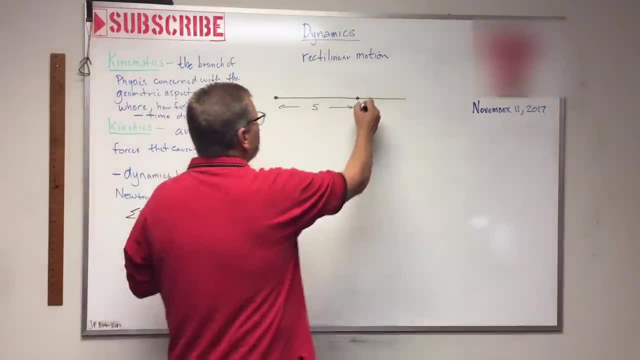 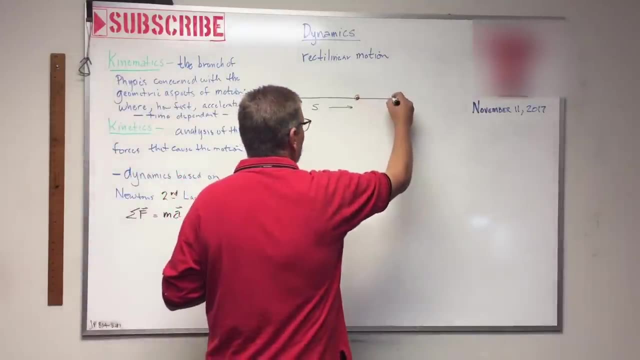 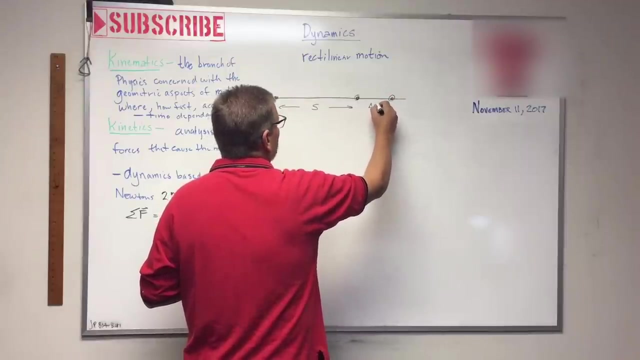 space. okay, so where is the location of our particle? this is our particle that we're concerned with now. let's say that particle moves some. okay, it goes from that position to, maybe, this position. so he moved. looks like eyeballs, doesn't it? okay, we'll put a little nose on him. no, let's call that. let's call that Delta s Delta. 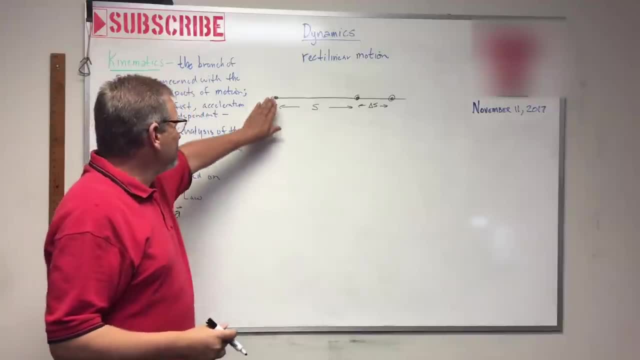 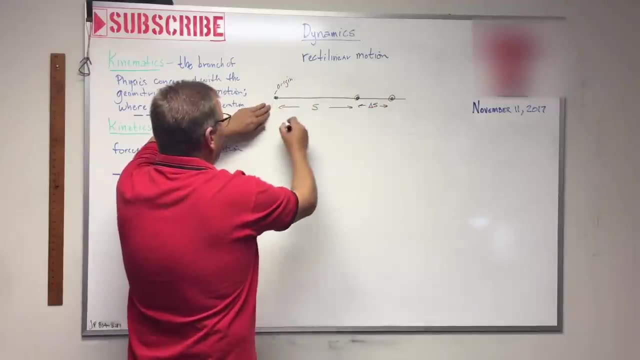 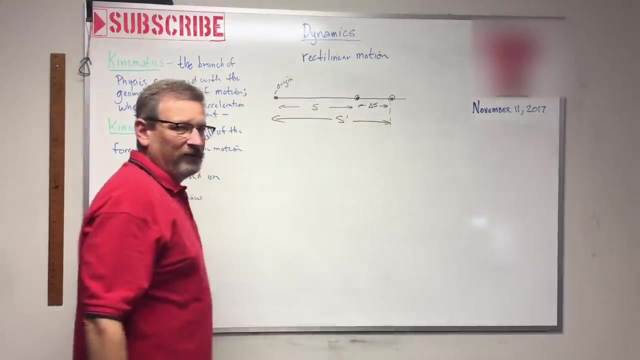 s is the amount that he moved. okay, so this is the origin over here origin. okay, then, that over there is this final position. okay, so we'll call that like s prime, which is his final position. so s prime is equal to s plus Delta, s or Delta. 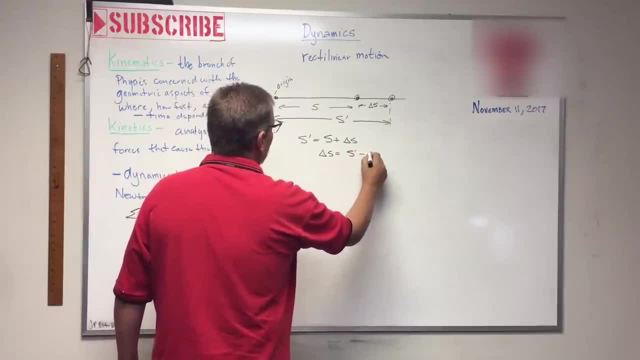 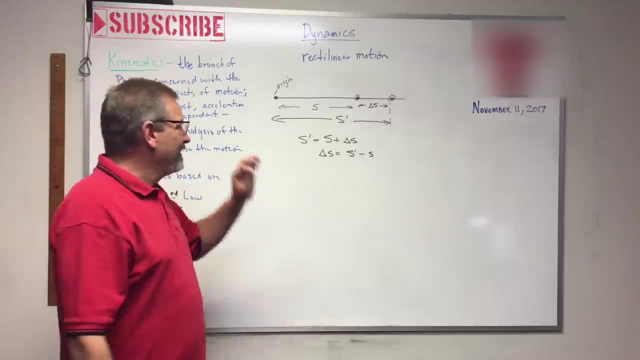 s is equal to s prime minus s right, either one of those works. that's pretty easy to understand, right? and that's about position of the particle. so remember the position when I started writing equations. position is represented with s, not X that we're used to, so don't be baffled by that. okay, okay. so if we know, 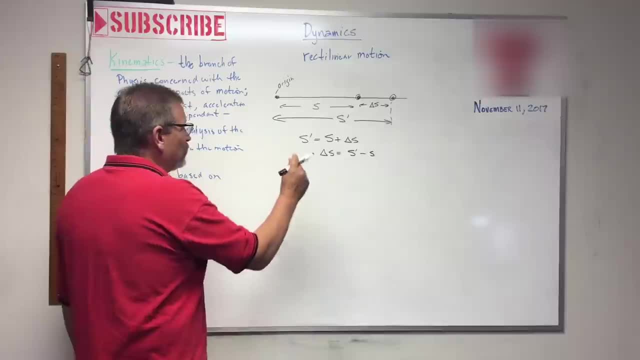 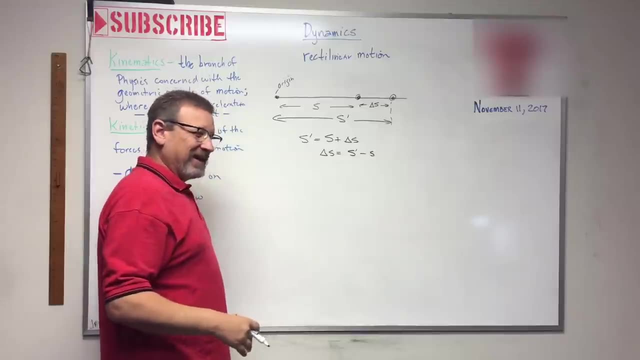 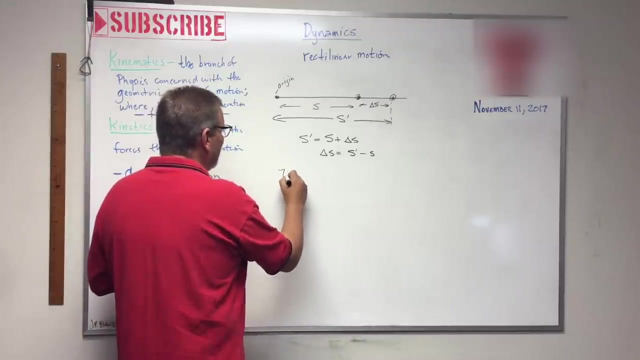 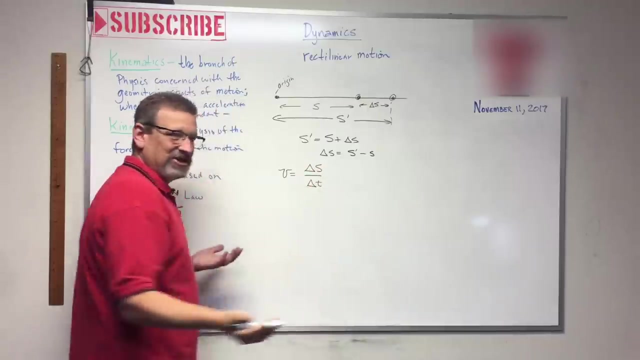 how long it took that particle to move from that point to that point, in other other words, how much time you know we could calculate, like how fast it moved over there, right, because we know the time and we know the distance, so we can say that velocity is equal to, like a change in position divided by a change. 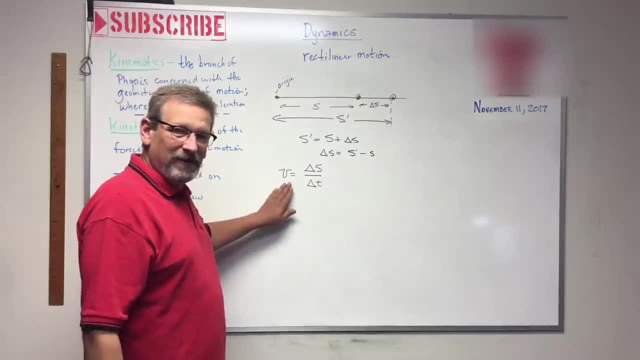 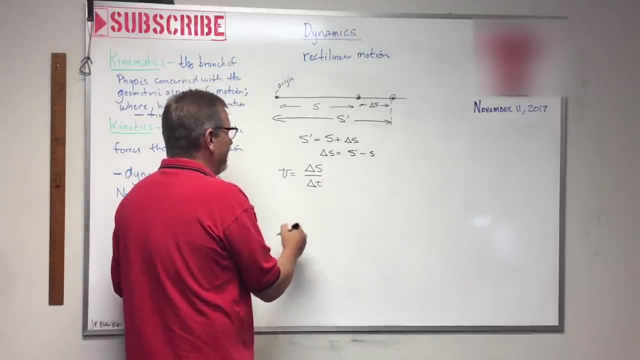 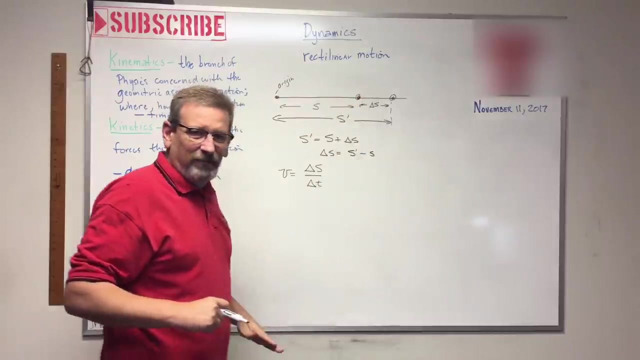 in time, and that makes sense, doesn't it? velocity is, like you know, in meters per second, so I'm moving so many meters per second some distance over time, you know. you know what we can do with this little Delta s. we could subdivide that into an infinite lump number of little tiny Delta s's. what would we call those? 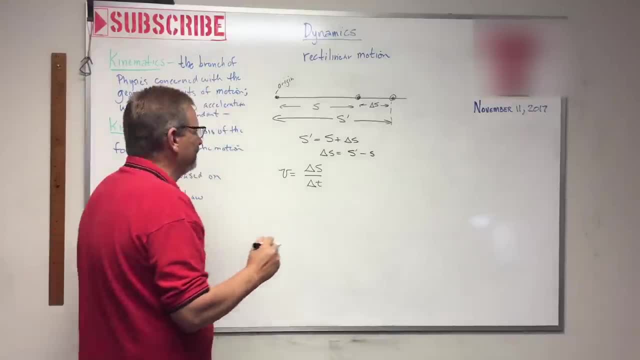 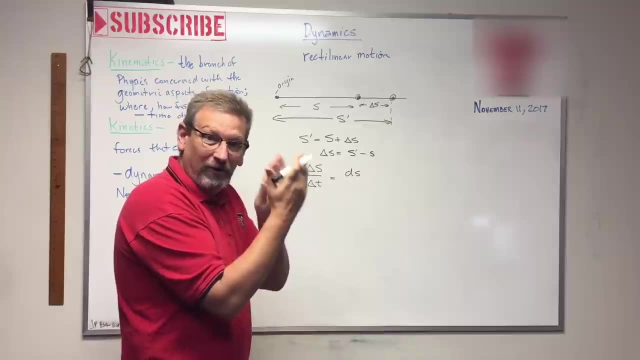 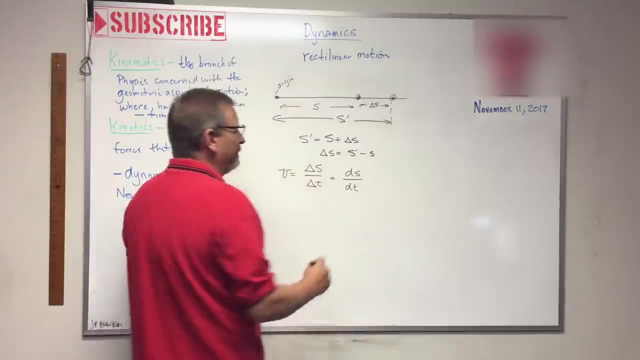 do you remember back from calculus what we call those tiny little Delta s's? we would call those little differential s's, right, every one of those little strips. remember in statics that are little differential areas. there's differential distances divided by those little differential times that go with that. 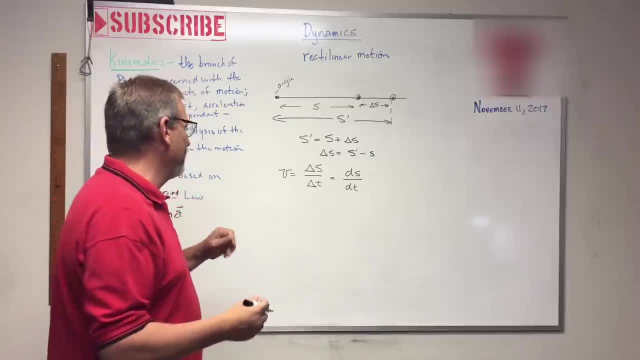 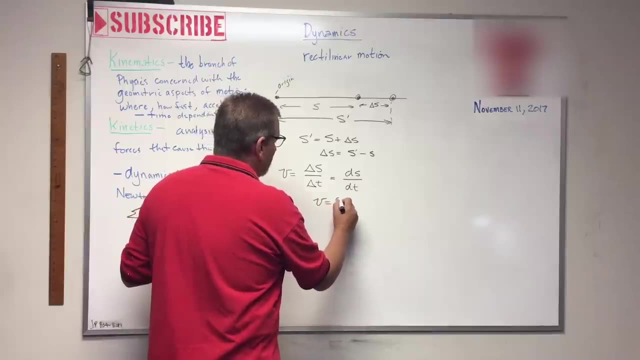 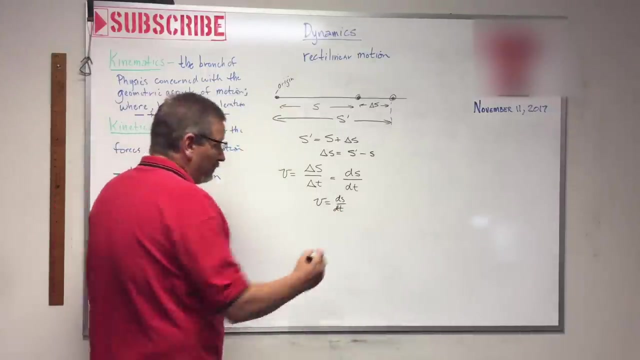 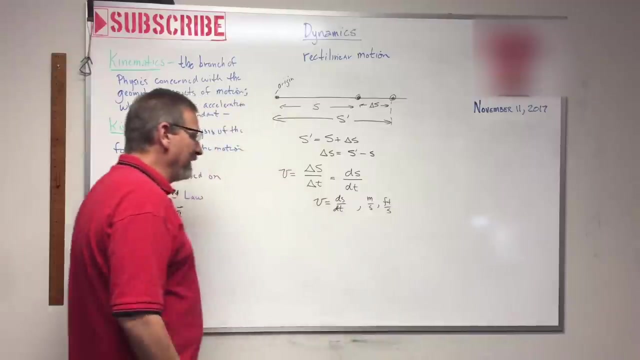 okay. so yeah, I guess there's going to be some calculus and dynamics, okay, and so what we come up with is this: this relationship here is that velocity is equal to DS over DT. okay, and again, the units for that might be something like meters per second or feet per second or feet per minute, you know some kind of a. 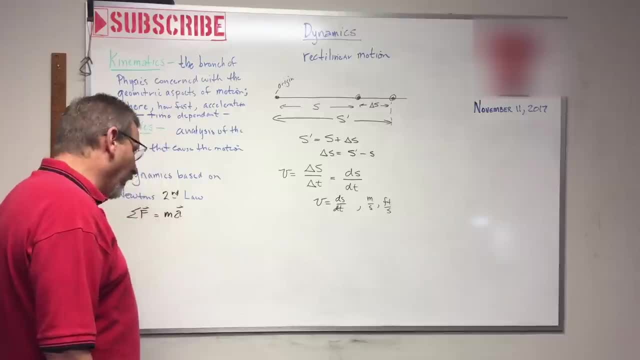 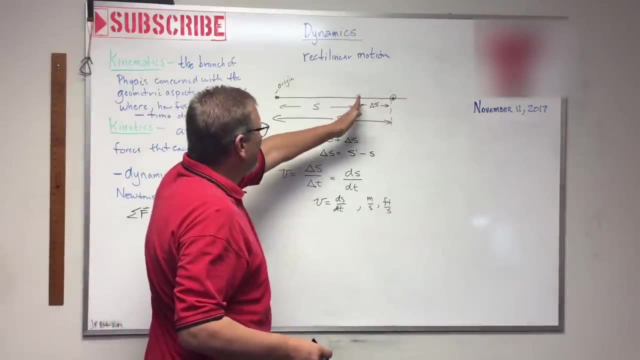 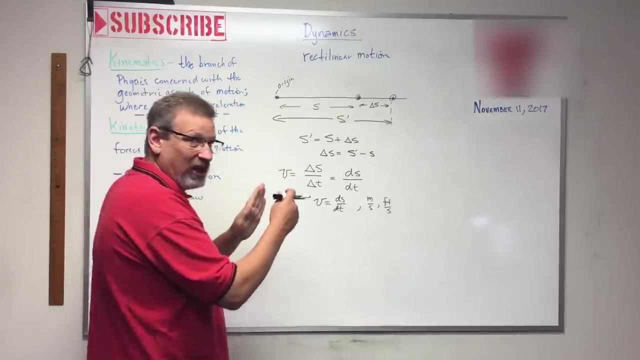 velocity unit there. okay, so also, if we know, we could know the velocity at two points, which means like we knew how fast it was moving there and we knew how fast it was moving there, then we can also have calculate how fast it accelerated or it changed. you know the change in velocity. 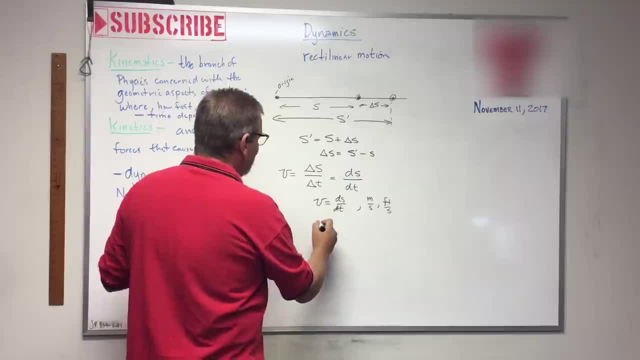 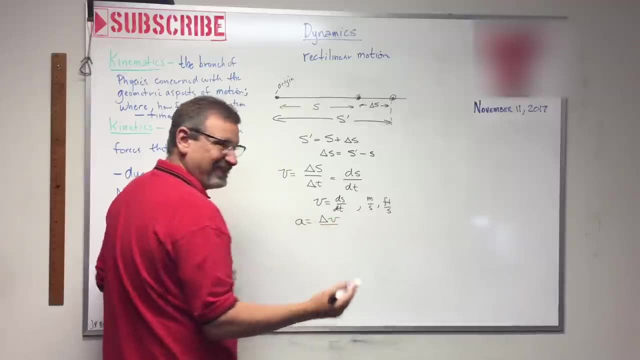 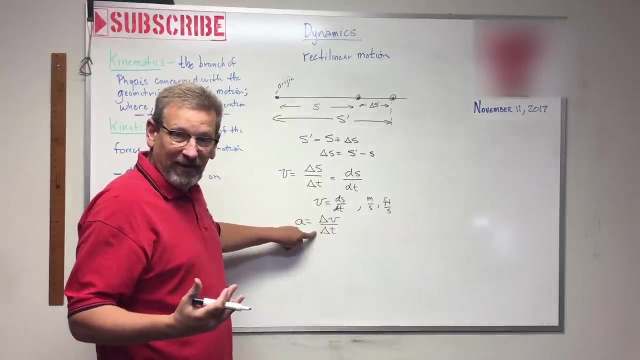 from one point to the other. so we could do this, we can do. by the same token. we can say: acceleration is equal to a little delta velocity, a change in velocity over that same change in time. right, How much did the velocity change over some period of time? 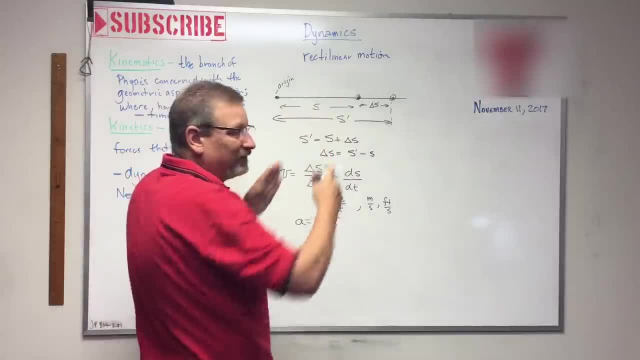 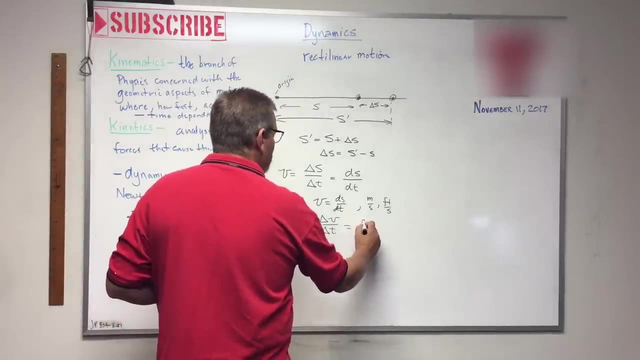 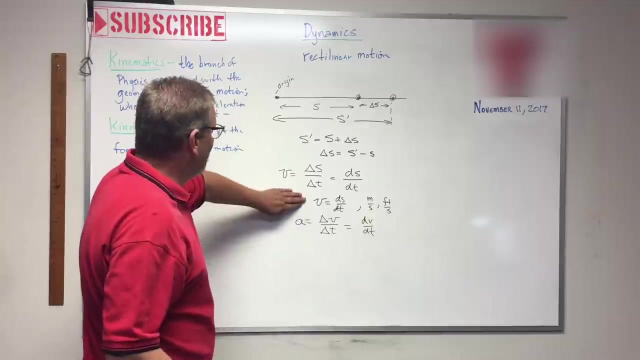 And again, if we started looking at little differential velocities in between there, right, we could get an equation that looked like this: that A was equal to dV over dt. okay, By the same way, we got this equation here. Now this is kind of a biggie, okay. 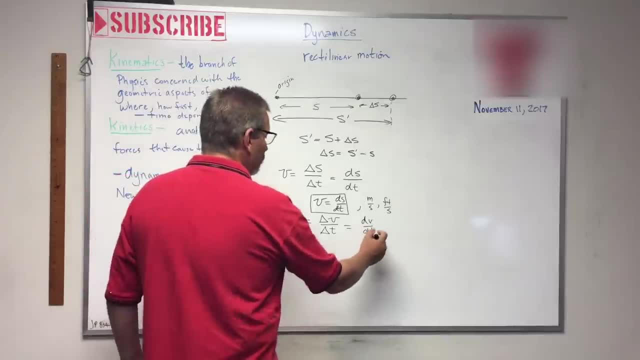 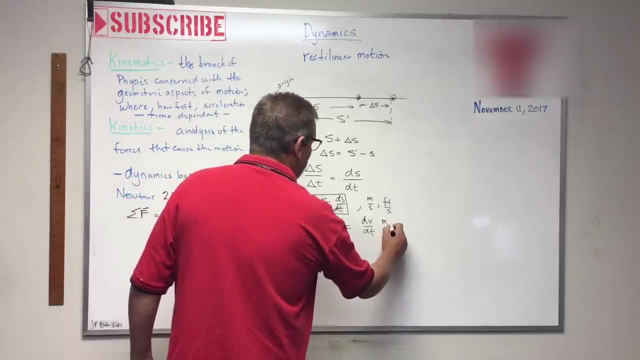 We'll put a little box around here And this one's going to be in. what is this? It's going to be in meters per second over time, so we get an extra time in there. So it's going to be like on meters per second squared this time, or feet per second squared, right. 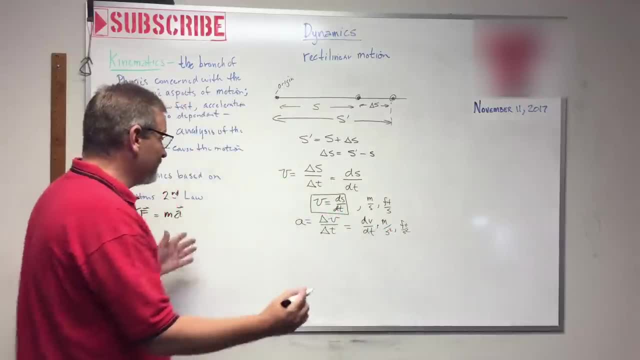 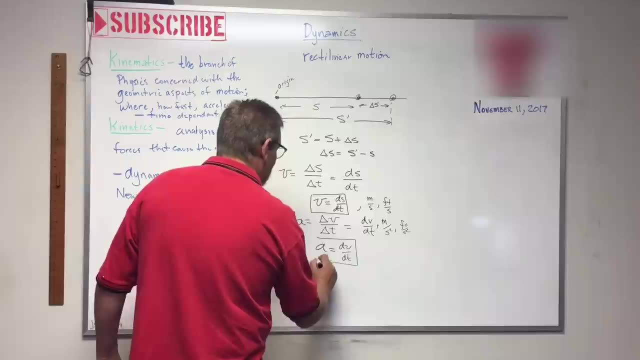 for the units for that guy. okay. So there's our next biggie. equation is A equals dV over dt. okay, Now, that's a biggie. Now let's just for instance: let's do one more, Let's get one more. 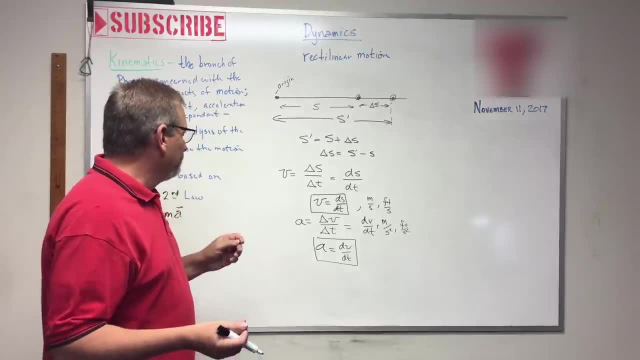 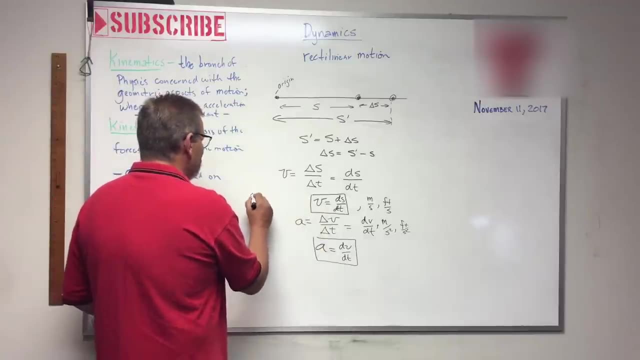 Now, this is not going to be a new equation, but it's going to be one we can get from this. Let's solve this guy for dt and this guy for dt. So we get. what does this one get? dt is equal to move that over there. dS over V, right. 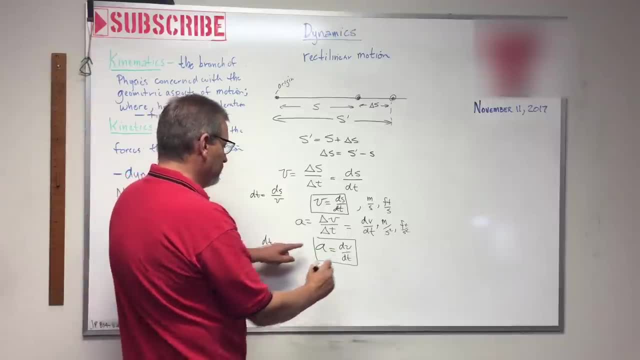 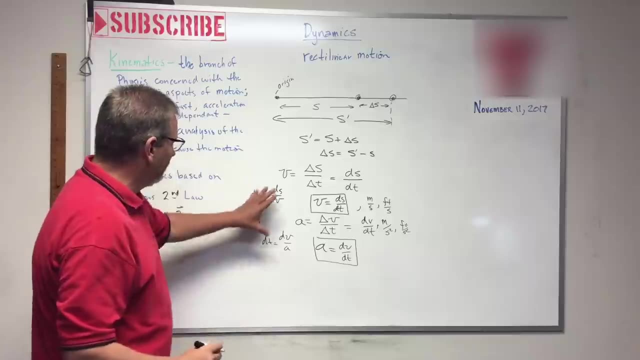 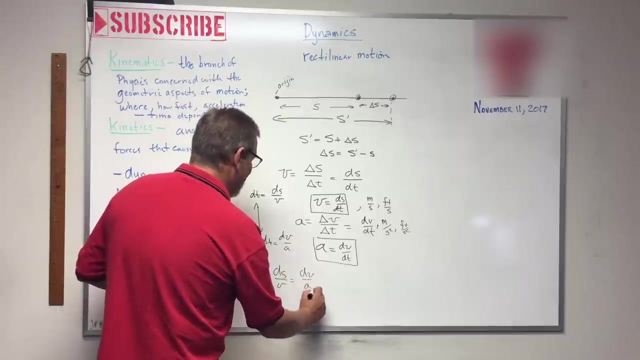 And then this one would be: dt is equal to move that over there, dV over A. And then we could set these two dt's equal to each other and we'd get this: dS over V is equal to dV over A. 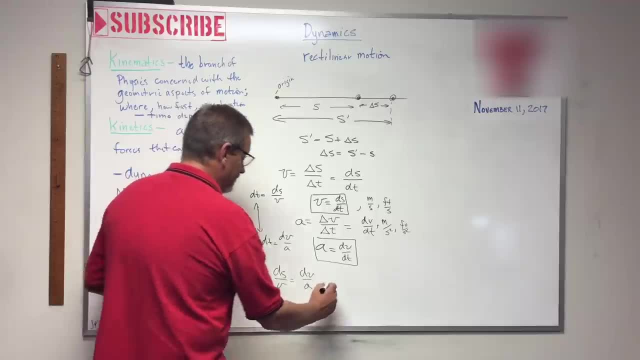 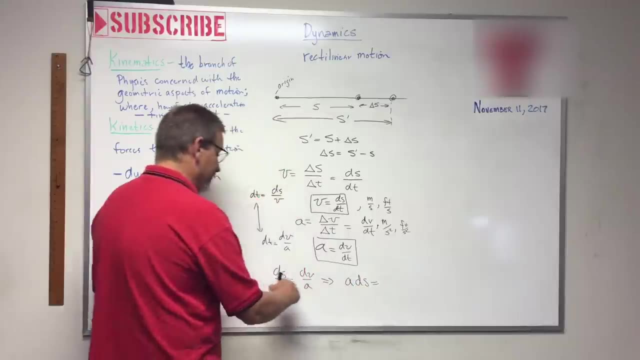 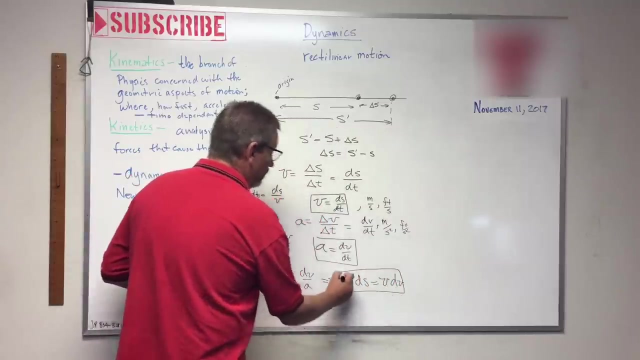 And then let's just solve that out. Move that over here, move that over there, so we get this. A dS is equal to what vdV, right, Okay? So that's kind of another big handy equation to have that relates acceleration to velocity, okay. 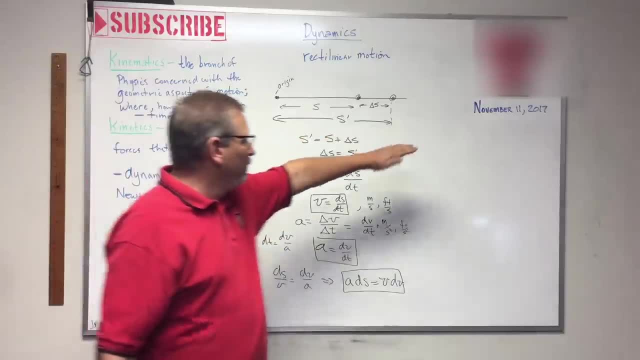 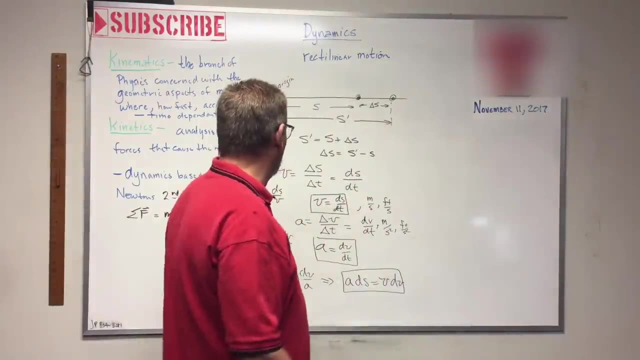 So these three are biggies. Let's put them over here, and as I go through the videos, I'll leave these equations over here so you can kind of see, remember those equations and follow along here. So these are the big ones that we've got so far. 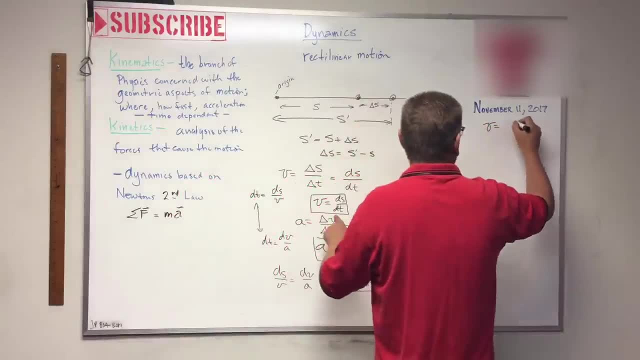 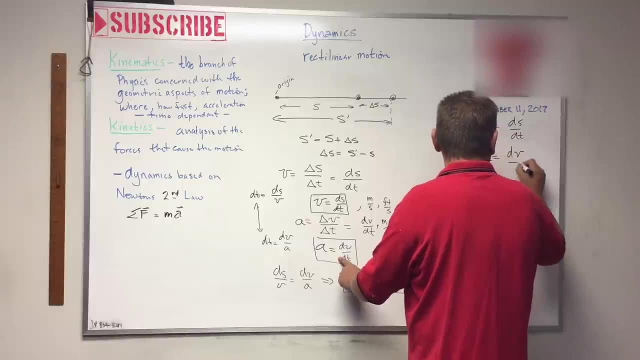 We've got v equals dS, dt and A is equal to dV, dt. and then this guy right here, A dS equals v dV. Now we don't have three equations here, gang. okay, Yes, there are three equations: one, two, three. 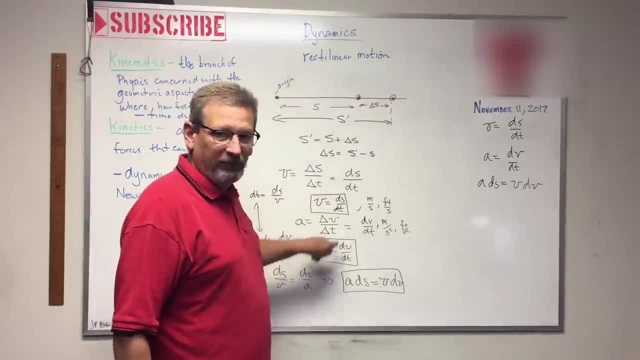 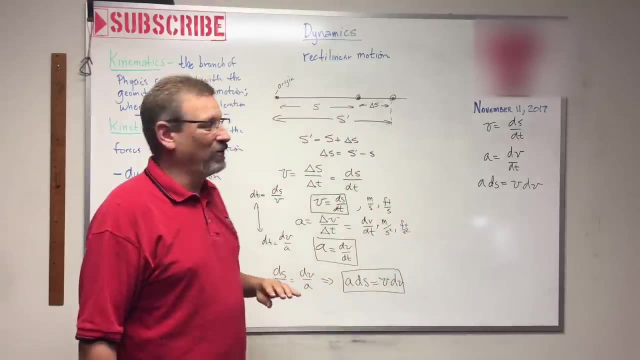 But this guy right here was just a substitute. There was no new information here, right, This one was derived by just substituting these two. So I can't like say, oh, I can solve for three unknowns now because I have three equations. 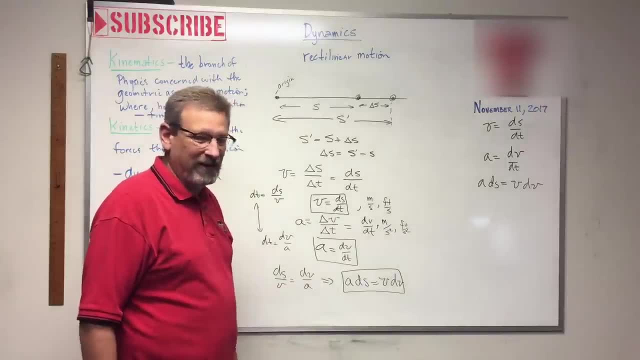 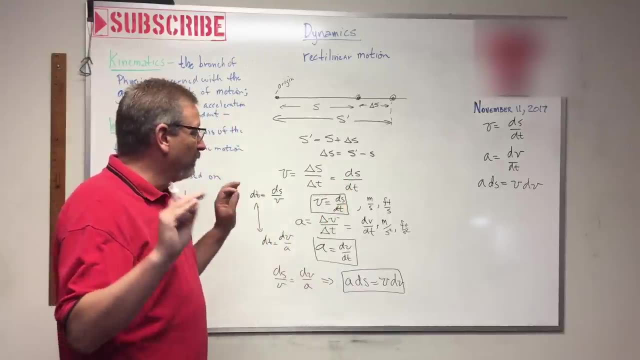 I really only have two, because I just substituted one into the other. okay, Now we're going to take these equations and we're going to do a little integrating and we're going to see if we can come up with something. Now, one of the things about these equations is: 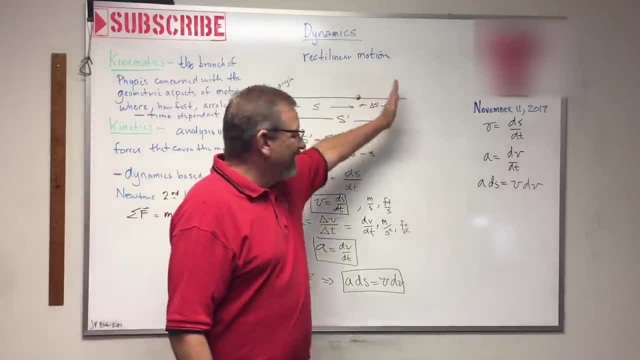 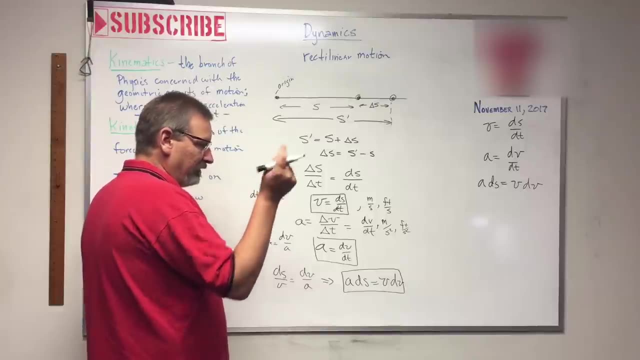 is this: acceleration from that point to that point was constant. That's important, okay, And if we use that information, we're going to be able to derive some new stuff. So let's erase this and let's keep going here, okay. 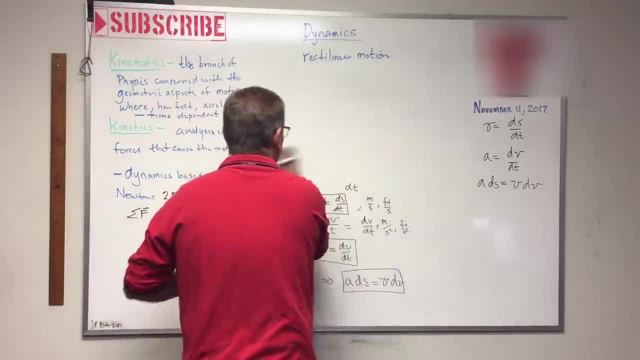 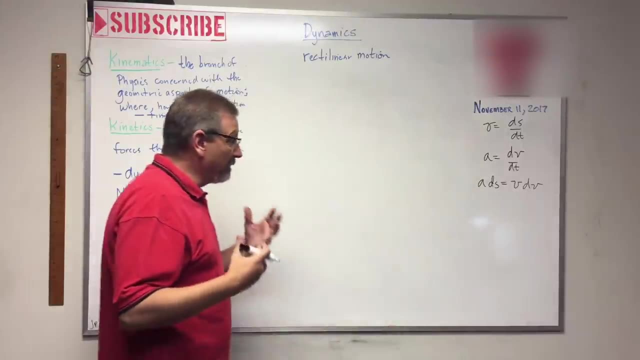 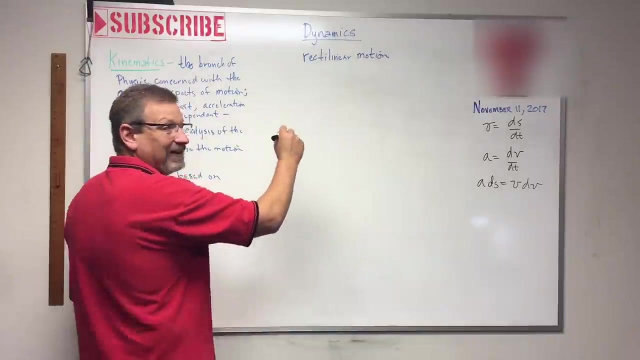 So let's get rid of all that, okay. So all we're doing is kind of introducing this rectilinear motion and kind of coming up with some equations that we can use to solve some simple dynamics problems, okay. So next let's take that equation and let's just see if we can integrate that. 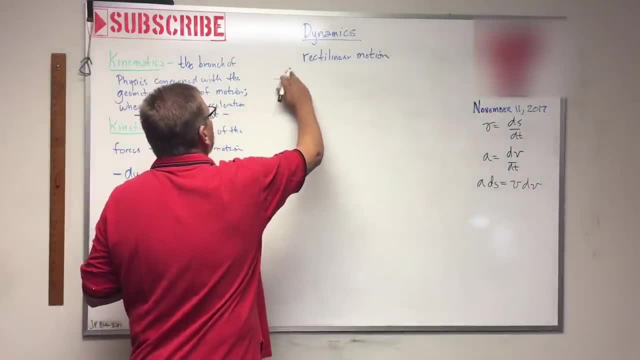 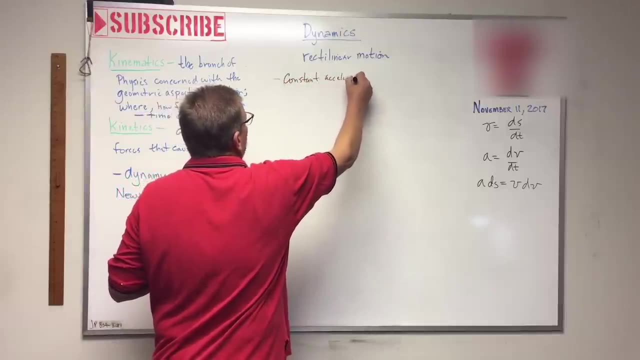 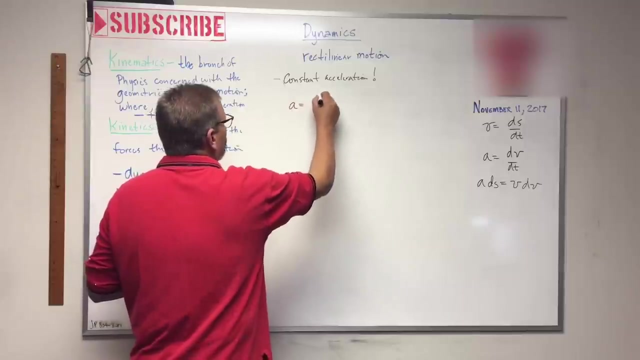 Now remember: this is important. This is important. This is for constant acceleration. That's important, okay, So let's take that equation A is equal to dv over dt And let's just get rid of the dt. Let's move him over to the other side. 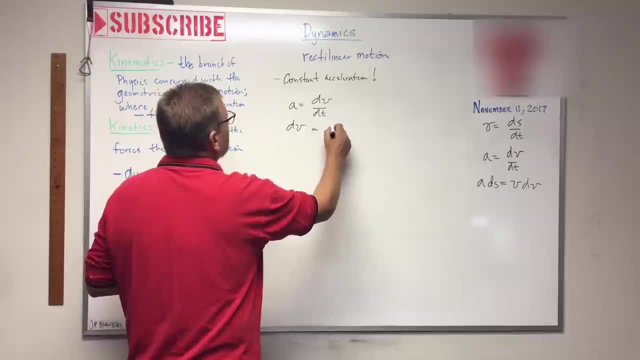 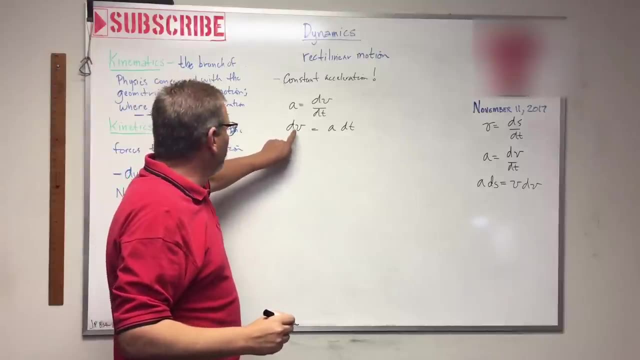 So we can get rid of the dt. So we can get rid of the dt. So we get: dv is equal to a times dt. okay, Now to get rid of this, let's integrate. Get rid of the little differential there. 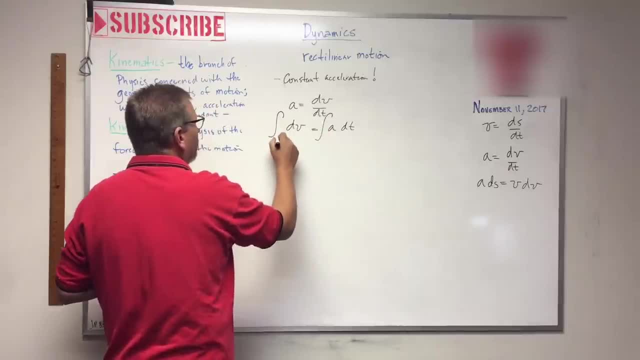 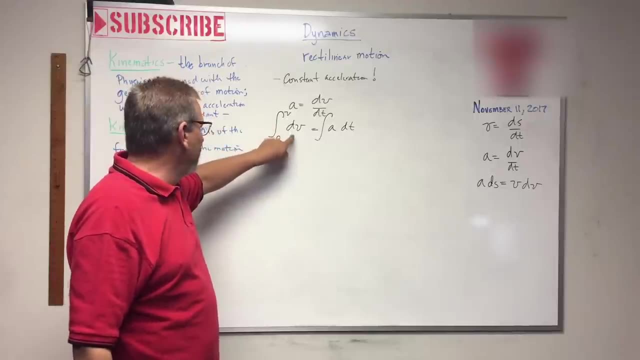 So let's just integrate both sides. Now, this one we're going to integrate from 0 to v. We're going to assume that this velocity was 0 when it started off, and there's this final velocity right And on this side we're going to assume this. 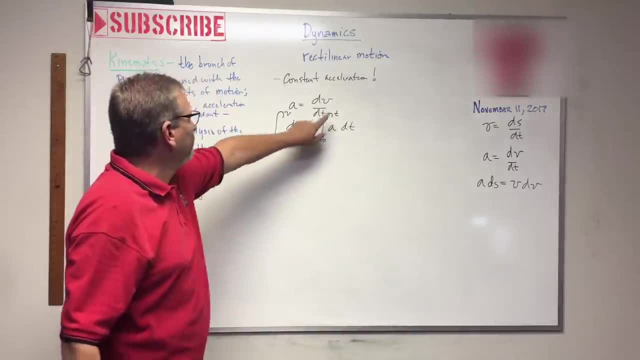 Time was 0, and there's our new time. okay, So we're going from 0 to t, 0 to v over here, 0 to v over here, And we're going to get this equation. We'll integrate this. 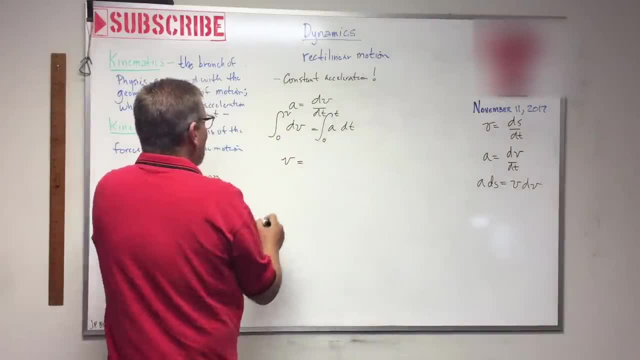 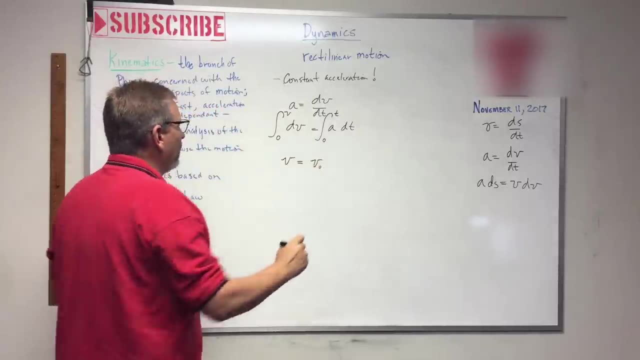 This: we're just going to get a constant right, Just v, okay. And on this side, what we're going to say is we can get a v0 because, remember, at time 0, our v was 0, okay. 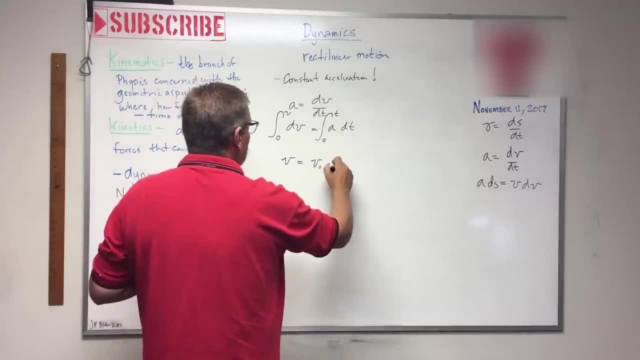 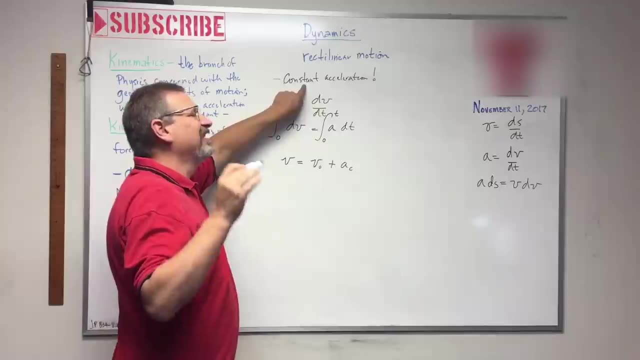 And then that is going to turn into what A is: just a constant. So plus a- and we'll put a little c there to remind ourselves that that's not just any acceleration, It's constant. okay, Times t. right, We get a t in there. 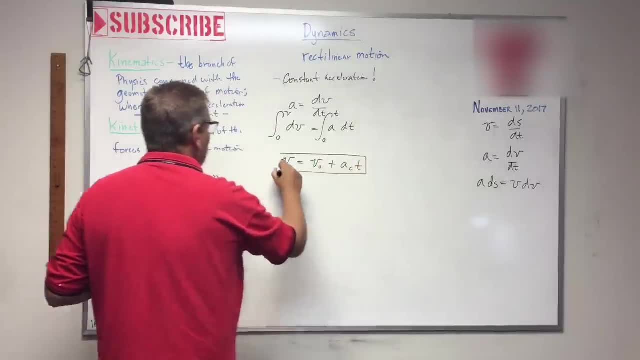 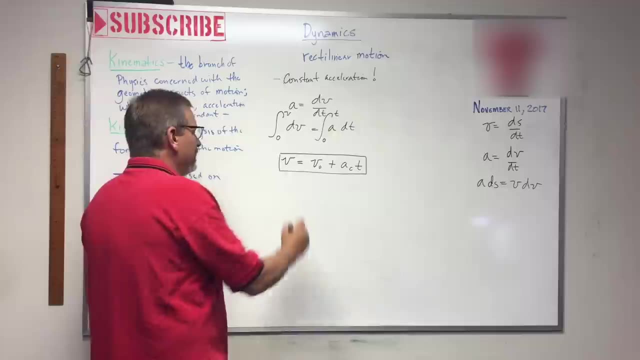 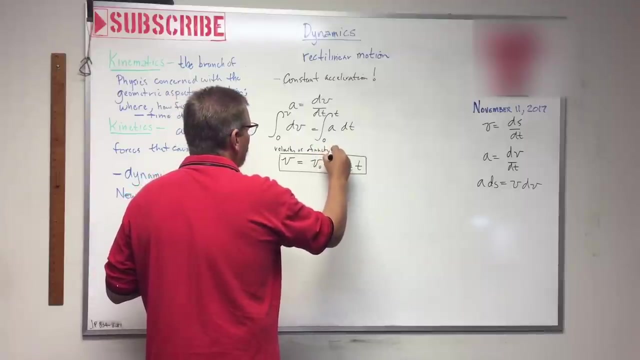 So there is equation number 1, okay, And that is going to be velocity as a function of time. okay, So this guy right here is velocity as a function of time. okay, So let's write that guy over here. This is an important one here. 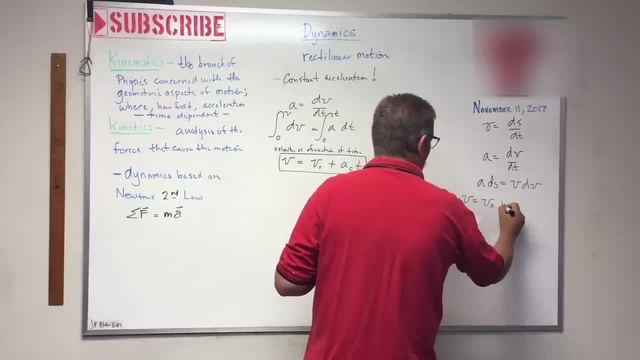 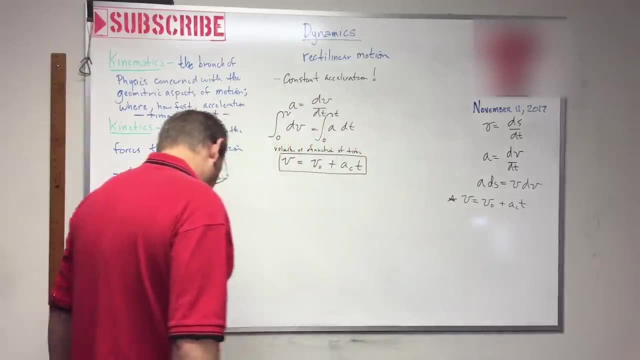 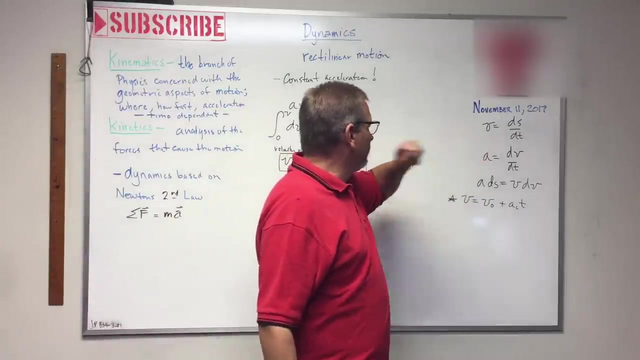 So v equals v0 plus a t. That's a biggie. okay, All right, All right. next, let's do the same thing. Let's take this equation here and let's see if we can integrate this one. 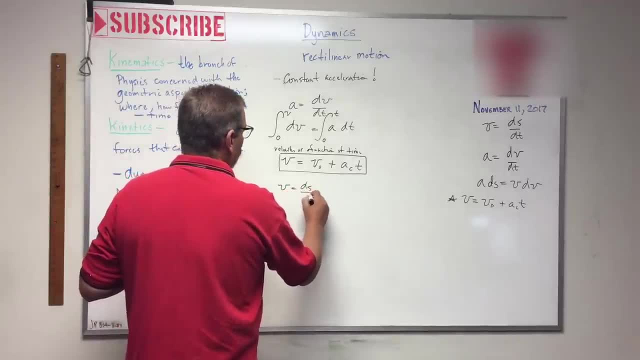 So we've got: v is equal to ds over dt. You know what? I know what v is equal to. I just solved for that. So let's do this: v0 plus ac. Let's take t and then let's move the dt over to the other side. 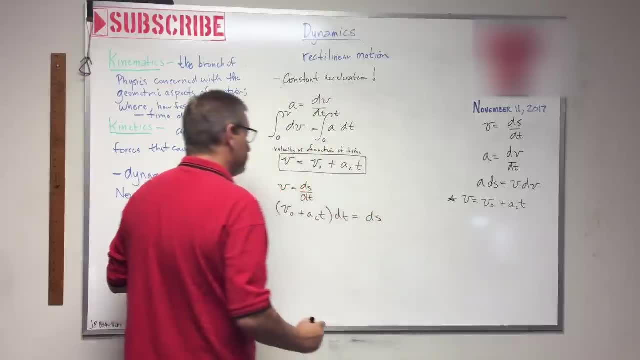 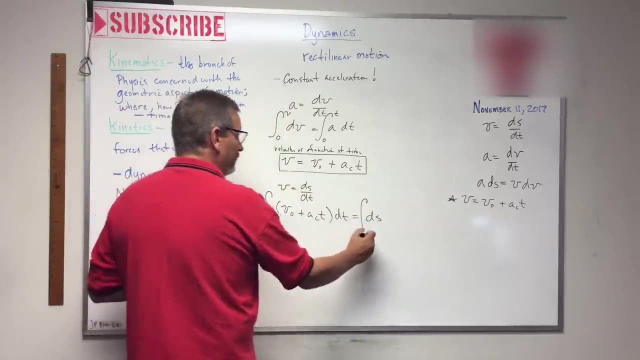 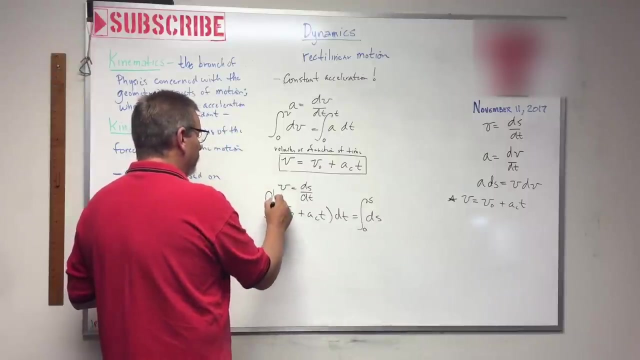 So dt equals ds. okay, Again, let's integrate both sides. This is position and this is time, right. So this is going to be from 0 to the new position s and this guy is going to be from 0 to time t right. 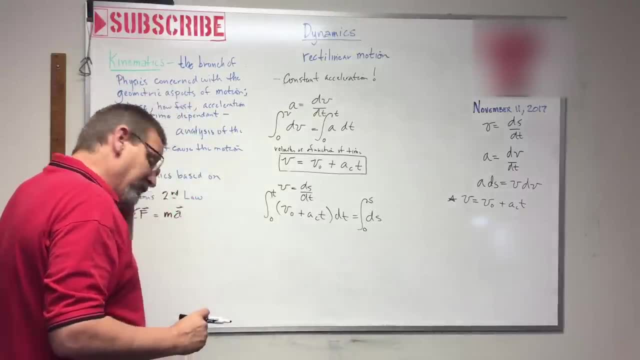 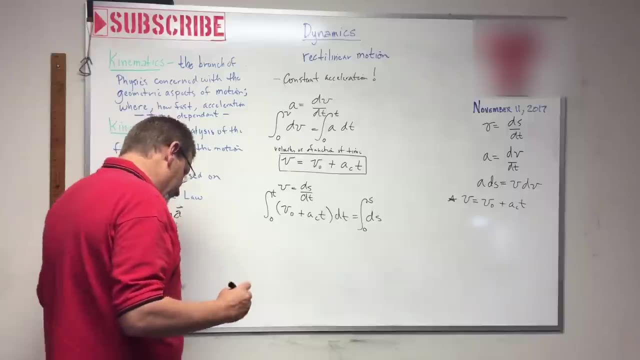 So this is a change in position. So what we're finding here is position, position as a function of time. okay, So we integrate this. We're going to get a new equation. This is a good one, okay. This side over here is just going to give me s, okay. 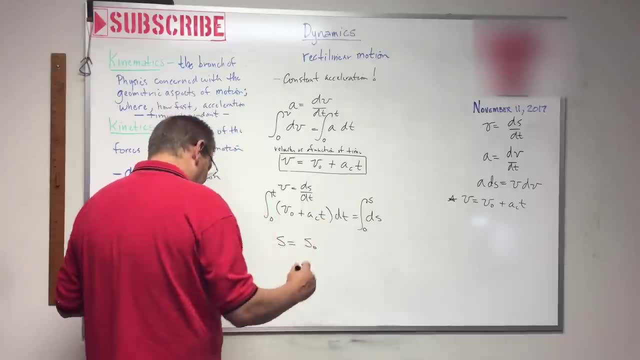 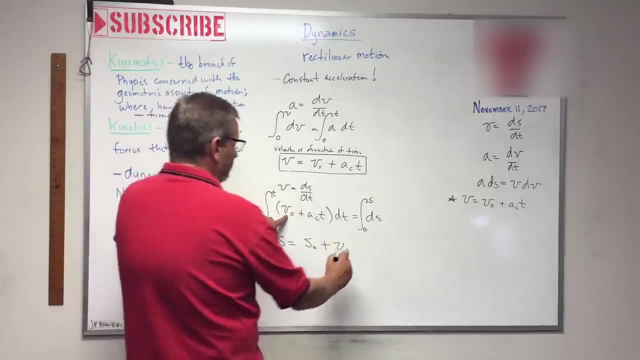 And this side over here is going to give me s0, which initial position again was 0, right Plus v0, and if I integrate a constant, it gets a t on the end of it, doesn't it? Plus? what's that going to be? 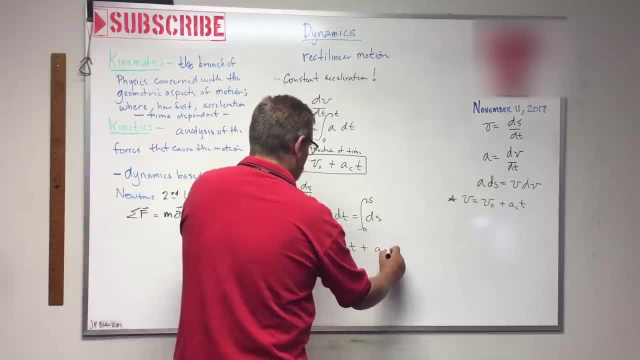 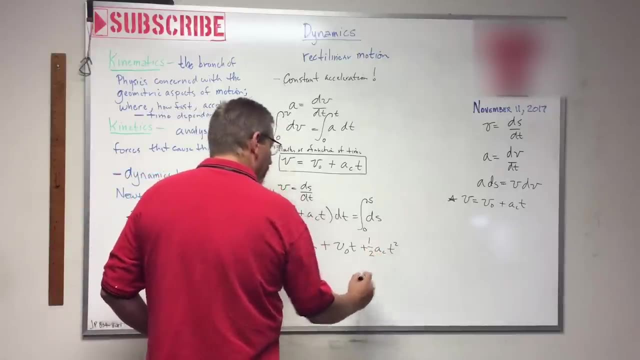 a constant t squared, A constant t squared divided by 2,, right? Or we could put a 1 half out in front of there, right? Because the t is going to give me a t squared over 2,, isn't it? 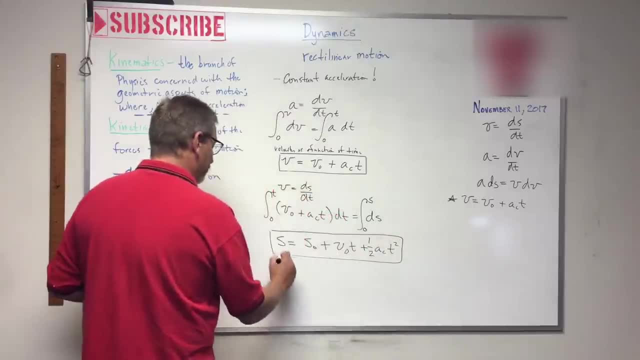 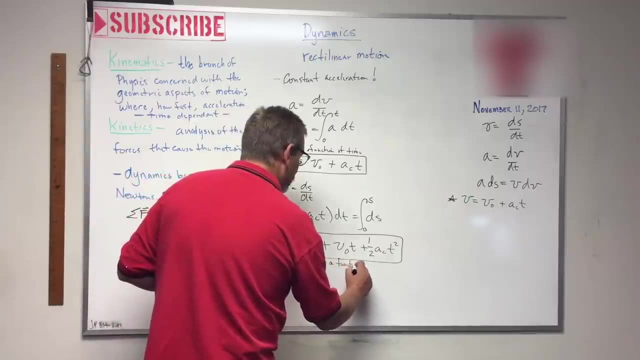 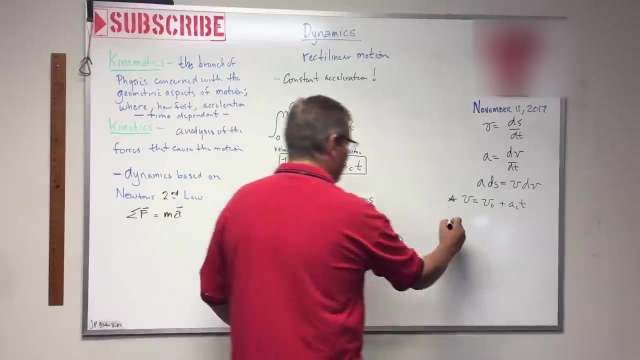 Bam, there's another equation. That's a good one. So again, this is position as a function of time. okay, Position is a function of time. Let's put that one over there. We'll put a star by him too. 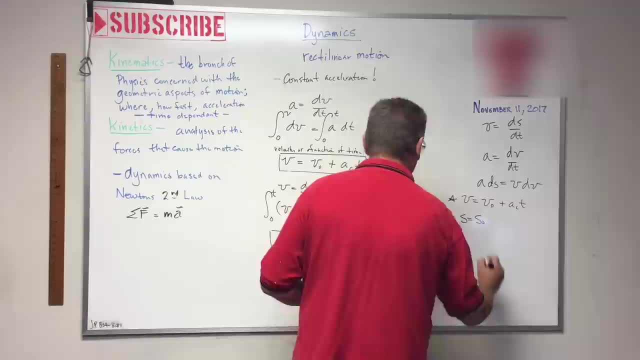 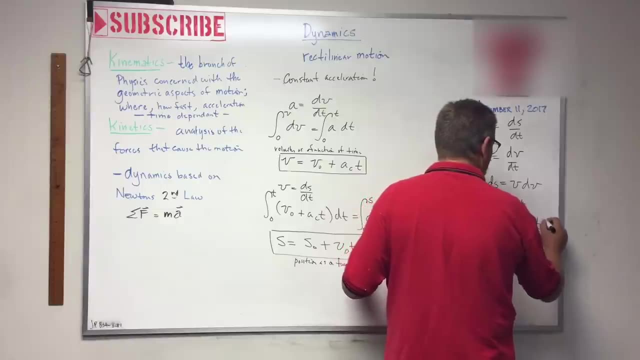 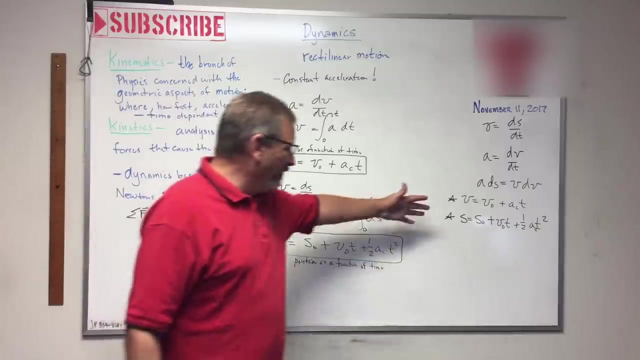 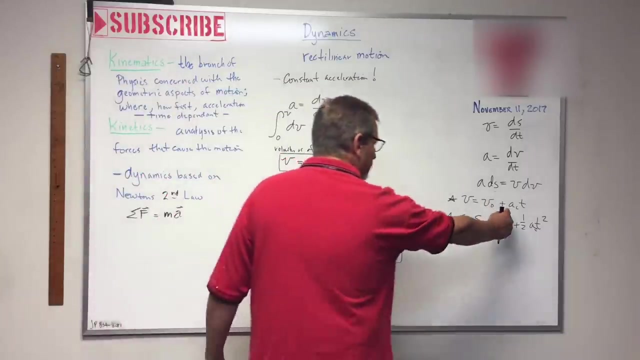 He's a good one. Okay, So s is equal to s0 plus v0, t plus 1, half a t squared Again, I'll put a little c there, because that's constant acceleration. We call these the constant acceleration equations. Now, from that, if I take this equation here and I solve it for t,